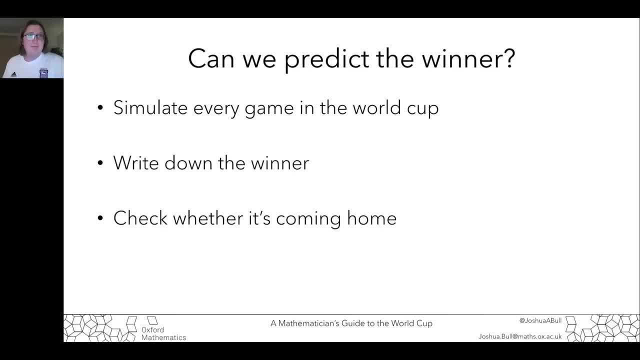 the end of that, I'm going to write down the winner of the World Cup And then I'm going to check whether that winner is England, which will be a good reality test for whether the model's working or not, And then I'm going to set the odds for England, which is going to be a very, very good 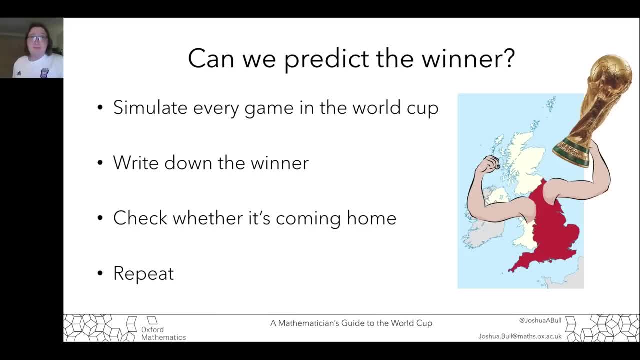 result, But the game is going to be a very, very good one, And I'm going to take the odds that it is coming home And I'll repeat this process many, many times. So the key thing is: we don't just do. 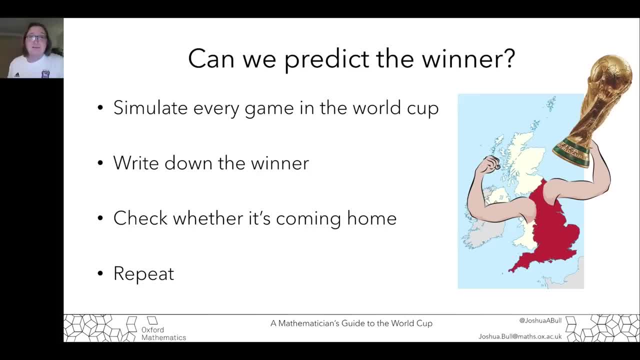 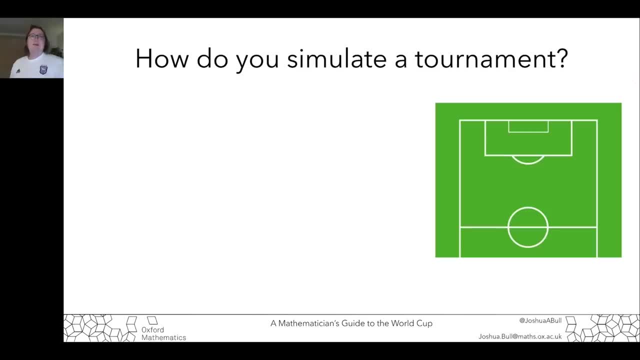 this once, because this is a very, very noisy game. Anything can happen in football. You know, it's a funny old world. But if we do this 10,000 times, 100,000 times, and we start to see the same. 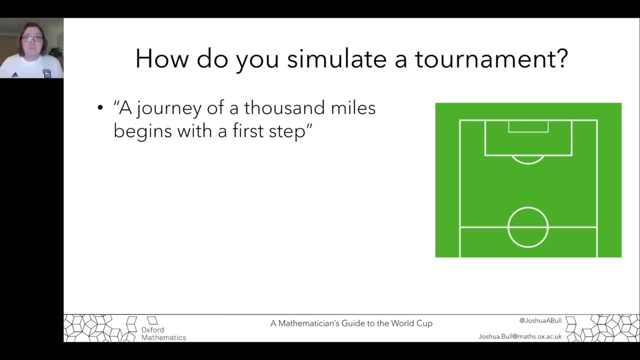 Well, a wise man, who I've forgotten to write down in this presentation, once said: a journey of a thousand miles begins with a first step And, as we all know, a tournament of 64 games begins with Qatar versus Ecuador. So let's take this one at a time. 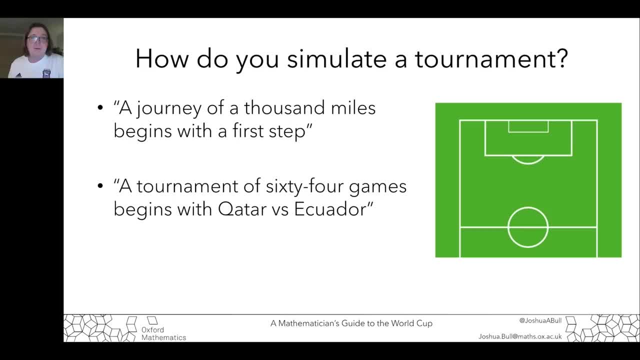 Forget about simulating the whole tournament. How do you predict who's going to win a football match? Is it just a coin toss between Qatar and Ecuador, Or can we use the information about which of these teams is better To make a prediction? 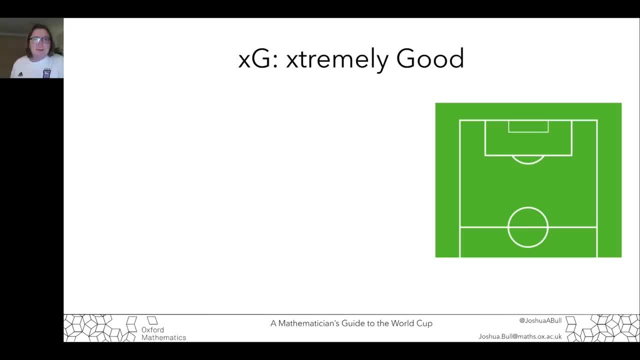 I think the answer is yes, And I think one of the best tools for doing this is something called XG, which is very popular in football modeling circles. So what is XG? Well, XG is a measure of how likely a shot is in a football match. 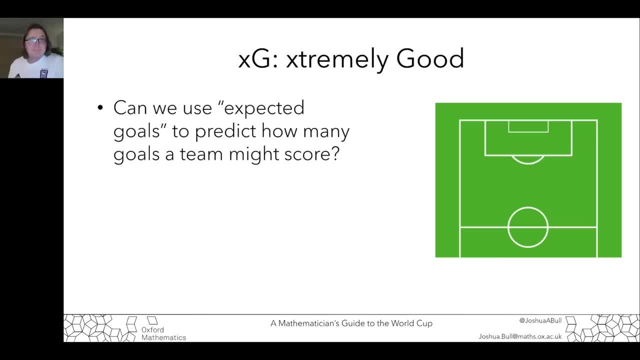 For a footballer takes a shot, what were their chances of scoring it? So this is a good measure for saying whether they were likely to score a goal or not, And it's great at kind of reducing some of the noise that you often get in football matches. 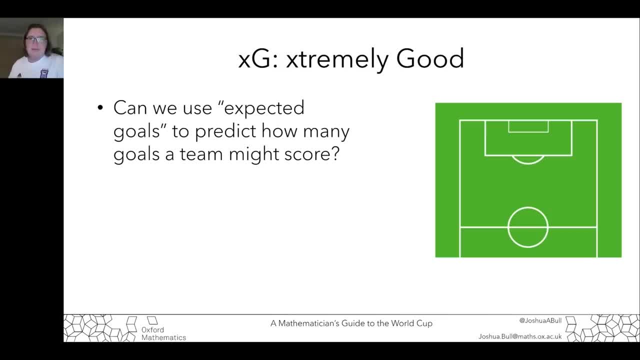 So sometimes a player might score a goal but they kicked it from the halfway line, The chance of it going in was one in a hundred and you know they just got lucky. And sometimes the team might do everything right And yet just you know, be really unlucky on the day and not get any points. 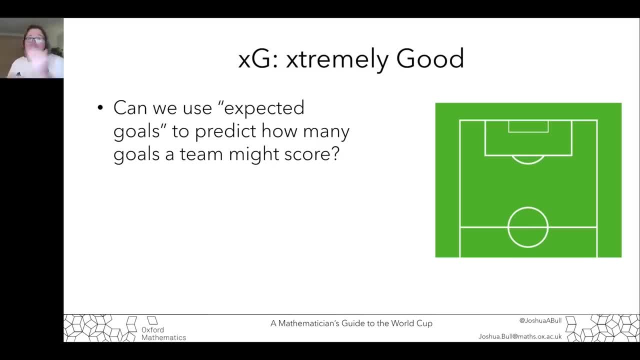 But there's still quality And maybe if they played that match again you'd see a different performance. So what XG does is, as a simplified form, it says: given where that player was and they take the shot, how likely were they to score? 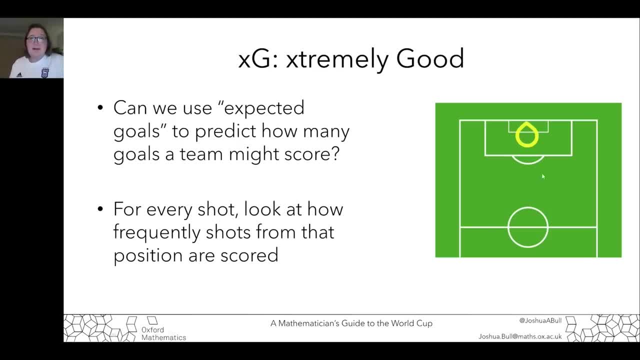 So if you're very close to the goal, where this little yellow thing is, you're much more likely to score than if you're taking a shot from further out or from further away from the goal. So this can, broadly speaking, give us a very rough measure of how likely a given shot was of going in. 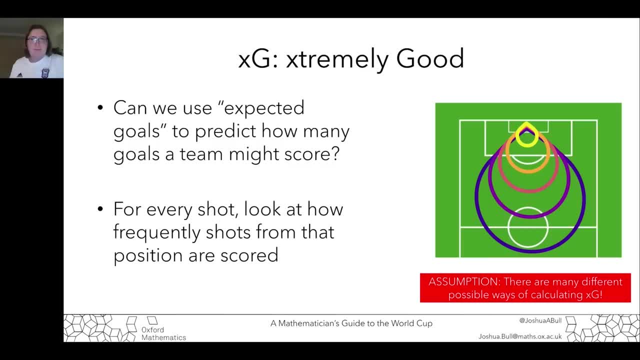 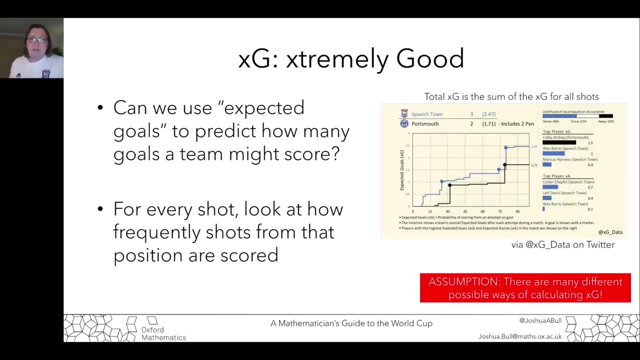 And you know we can add up all of the shots that are taken within a game by the England team, say, and we can look at how often they go in. So this is from the big Ipswich versus Portsmouth match a few weeks ago. 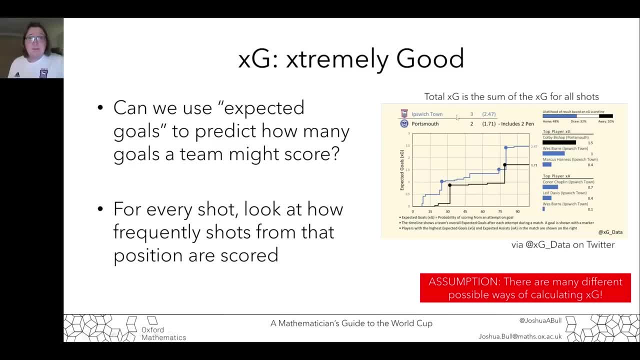 And you can see that the actual score was 3-2 to Ipswich. But when you add up all of the XG here, Ipswich had 2.47 expected goals and Portsmouth got 1.71, including two penalties which you can make your own judgment on. 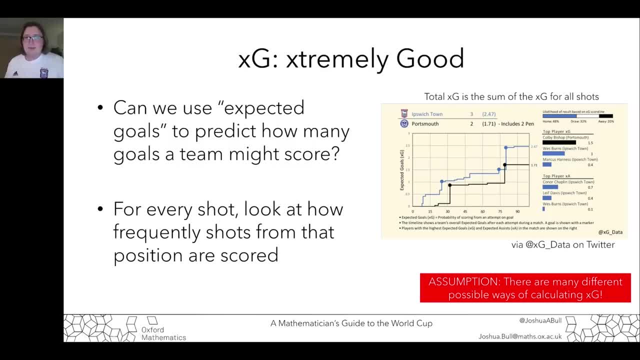 you know the relative quality of these teams. I will remain unbiased here. So the important number for predicting what this match would look like would be to look at this total XG that scored in this match And we can say, well, OK, maybe 3-2 wasn't such an unlikely scoreline. 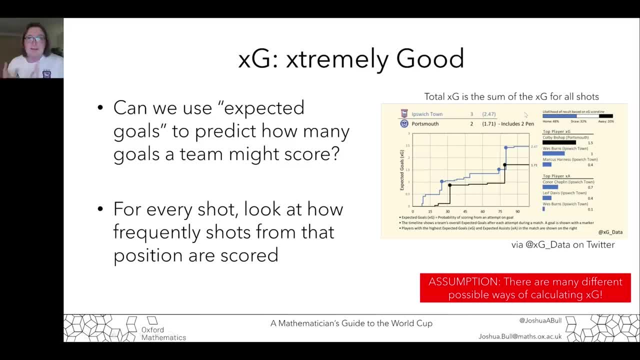 Maybe if this had been 5-0, we'd have said: yes, that's a bit unlikely, But it could still happen. So what we need is a way of going from this kind of predicted XG for the team to the score of a football match. 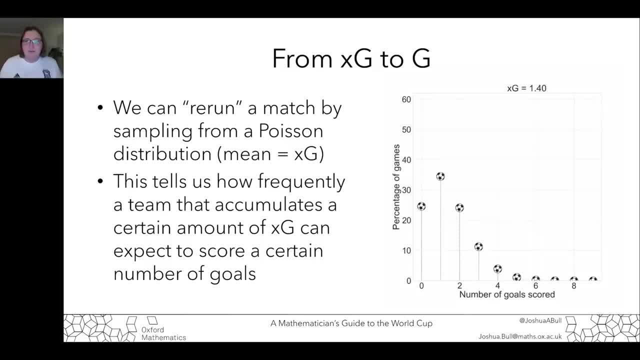 And the way that we can do that is by using a Poisson distribution. So this fancy graph that I'm very proud of because I managed to get footballs into matplotlib- Yeah, love it- This graph shows basically, for a given XG, how many games will have a certain number of goals. 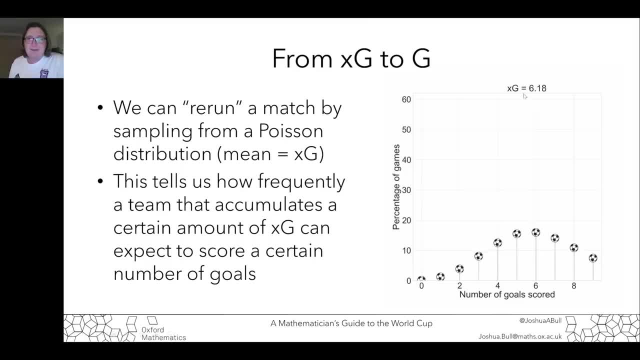 So at the moment we're looking at quite high numbers. If my team has an XG of around six and a half, then I'm expecting to see six goals scored by that team in as many as 20% of the games, And you can see as the XG goes up. 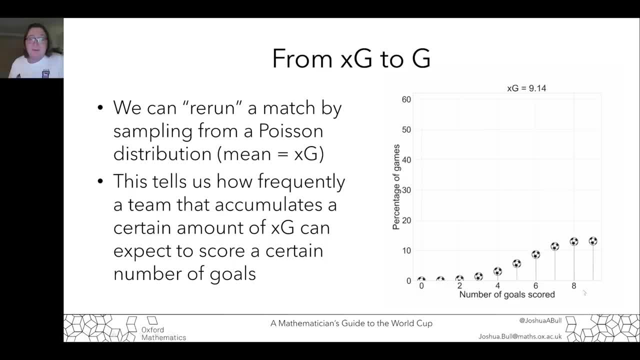 the total number of goals that that team's expected to score is going to go up as well, But obviously you can't score half a goal. So this is really telling us. if we look over a lot of matches, this is what we're expecting to happen a certain number of times. 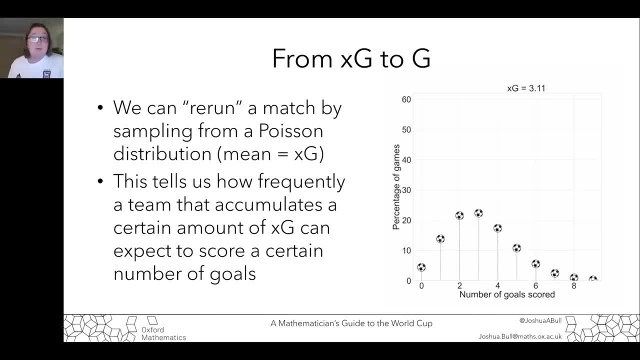 So low XG in most games. there'll be very few goals scored, but occasionally it's going to be higher And the Poisson distribution turns out to be a good way of modelling this. There are other assumptions that you can make. 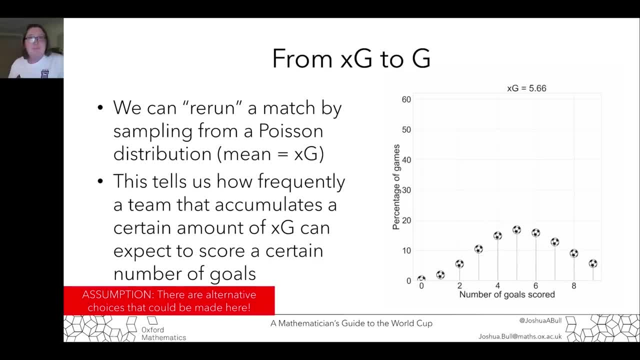 And this is a key thing in the process of mathematical modelling is: you make assumptions and you see what happens, And if That gives you believable results, then you say maybe they were good assumptions. If something goes wrong, that tells you where you can revisit and change what you're doing. 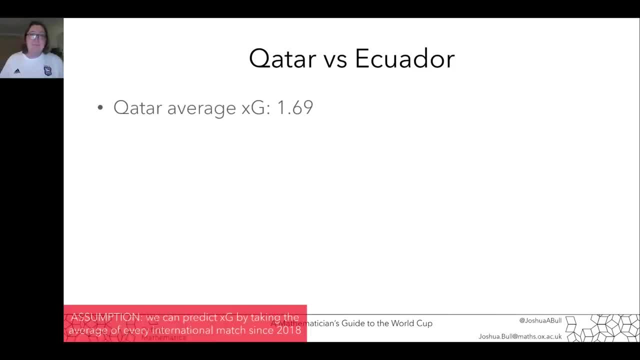 So back to Qatar versus Ecuador, the big game. Well, on average. if I just look at every international match that Qatar has played in the last four years, I know that on average they score 1.69 goals. That's their XG. 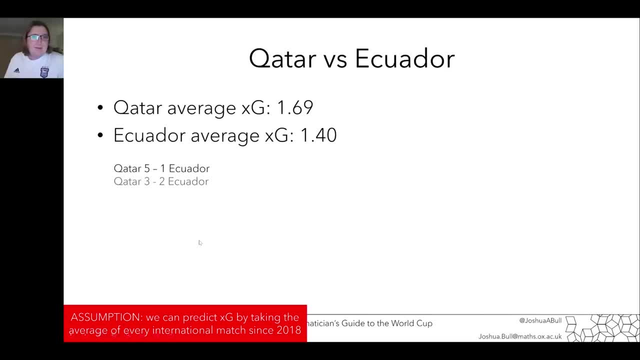 Ecuador, on the other hand, 1.4 XG. So I can use our Poisson distribution sample from two different Poisson distributions and end up with loads of simulated scorelines, And I'm going to put them in a funky heat map. 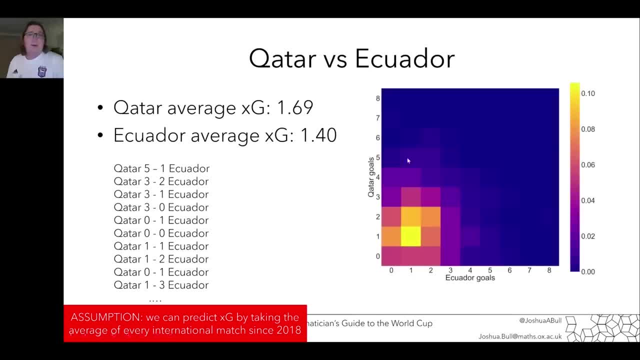 which basically shows what the expected distribution of the scorelines is. So you can see here, the most common score here would be 1.1.. But there's maybe a few more goals, a few more matches where Qatar is scoring more than Ecuador. 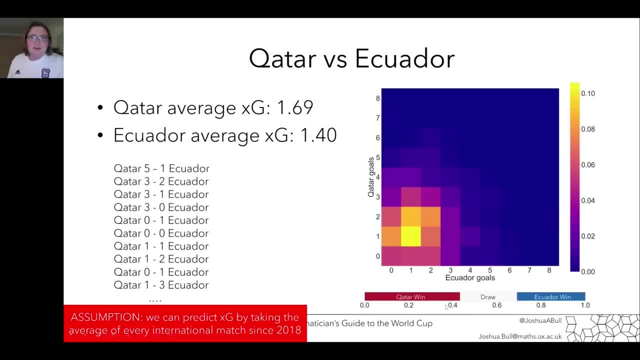 And I can say that, on average, under this model, Qatar are likely to win this about 45% of the time, whereas Ecuador are only winning maybe 30% of the time. So this is great. This gives us a way of simulating a match. 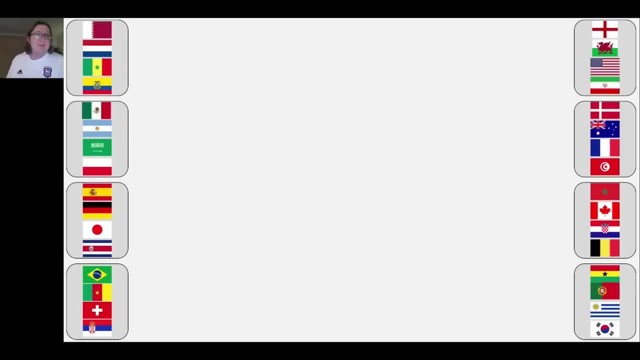 So let's go ahead with this kind of very simple model and see what happens with the World Cup So I can see who I think is going to get through the group stages from just running one particular iteration. Yeah, I'm not going to narrate all of this. 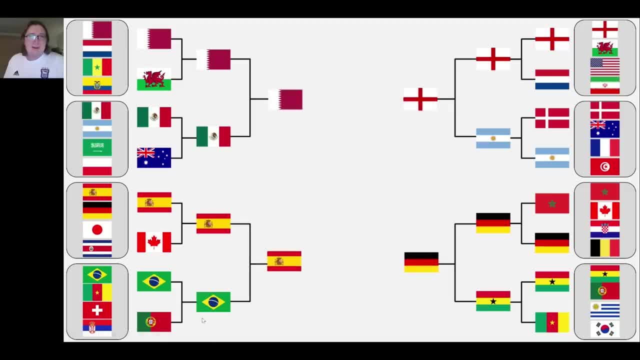 but you can kind of have a lot of fun watching the model kind of do some likely or unlikely matchups before we get to the big England versus Qatar final And by sheer chance, the simulation that I happen to use for this one has an England victory. 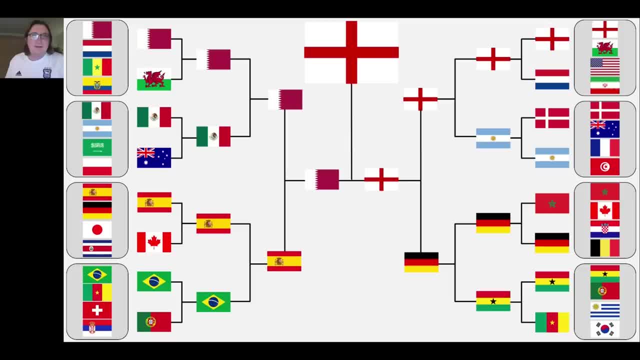 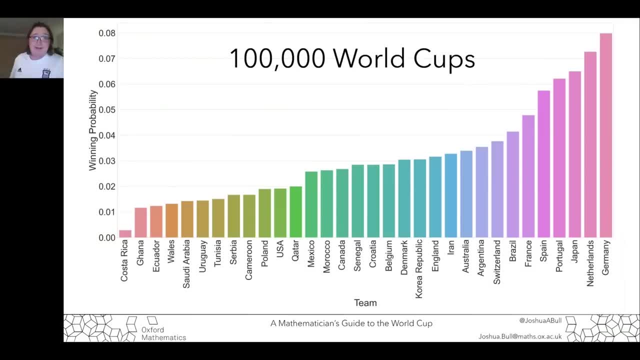 which you know, maybe it's just fate. I definitely didn't fudge that at all. So if I do it 100,000 times, unfortunately England dropped down the list a bit And you can see here that Germany and the Netherlands do very well here. 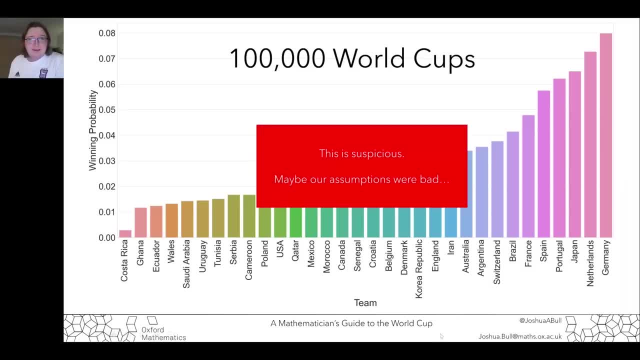 which we might expect, But it is a little bit suspicious, right? Because England are down here, just below Iran, and Japan are right up the top. Japan are winning the World Cup about six and a half percent of the time, according to this model. 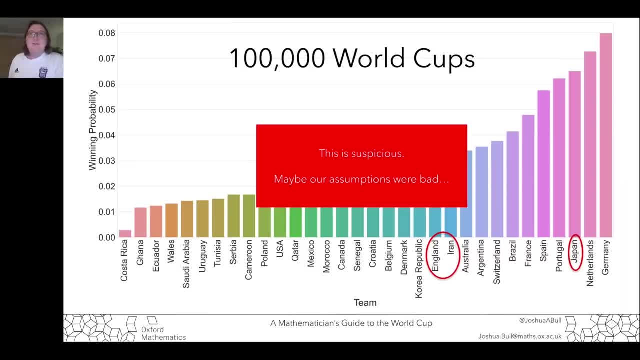 This doesn't seem very likely. So we say, well, okay, when our model is behaving in a way that we think is probably not realistic, that's maybe a sign that we're making bad assumptions. And the assumption that I'm going to look at here is the idea that I can predict. 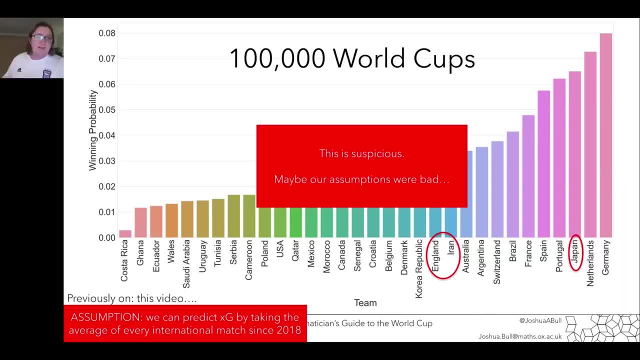 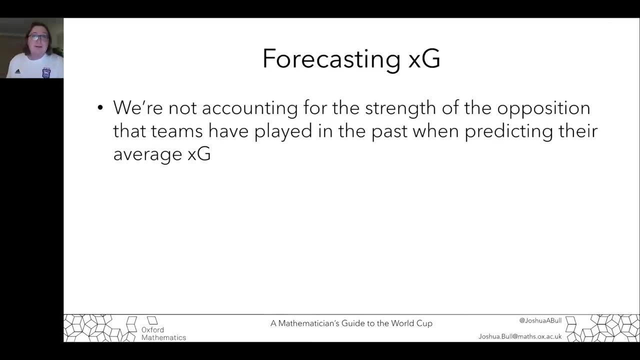 what England's XG will be by just averaging what they scored in every previous international match. That's their XG- sorry, not their actual goals- And I've been looking at the last four years. but this maybe isn't a good way of kind of predicting this, because obviously 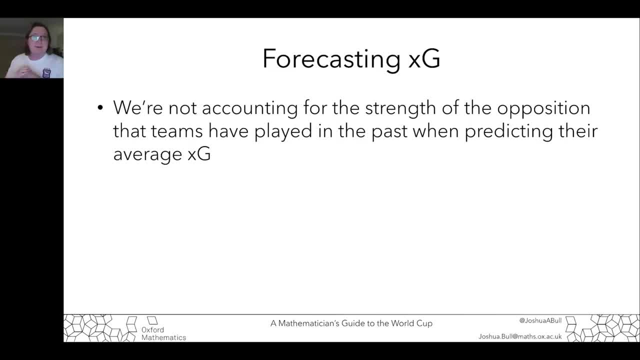 the XG isn't just a property of a team. It's a property of who they're playing. If I'm playing against a really, really strong opposition and I don't get very many shots, I'm going to have a very low XG. 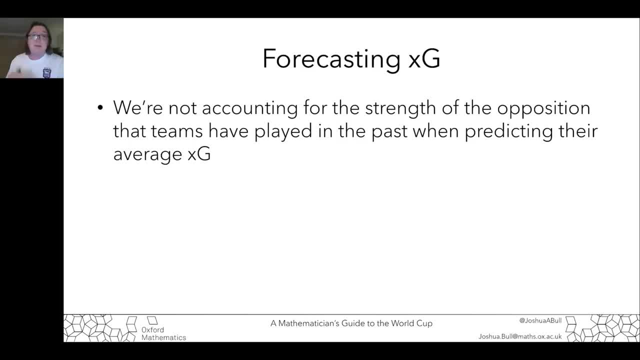 Whereas if I'm playing against very weak teams that maybe don't defend as well, maybe I can get incredibly high XG despite not being a good team, And that's exactly what you see when you look into the data. So, for instance, Japan: 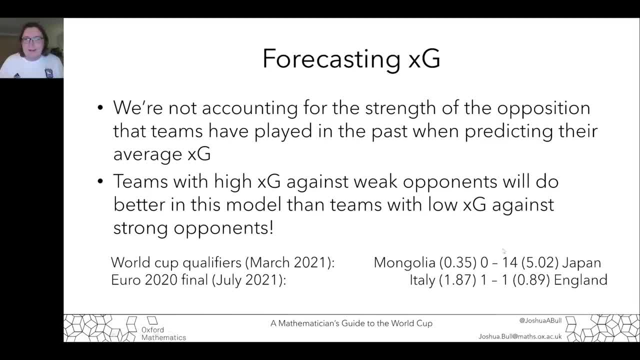 who were coming out very highly on our model, have had several matches like this, Mongolia versus Japan, where they managed to win by a colossal amount of goals, racking up an XG of 5.02, which is pretty huge, Whereas England have had some tougher matches. 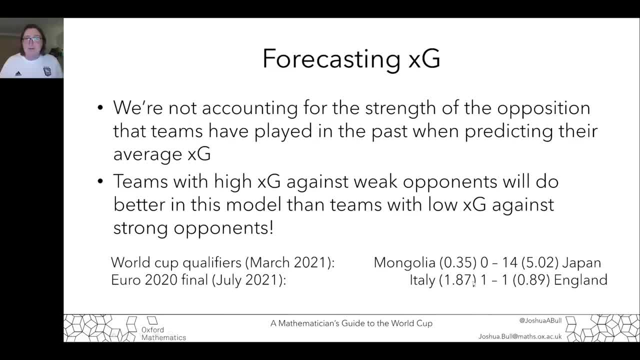 So, for instance, playing Italy in the Euro 2020 final- and, yeah, everyone will be a little sad- Well, I say everyone, but maybe not the Italians- to see that actually, Italy probably deserved the win there. They scored twice as much. 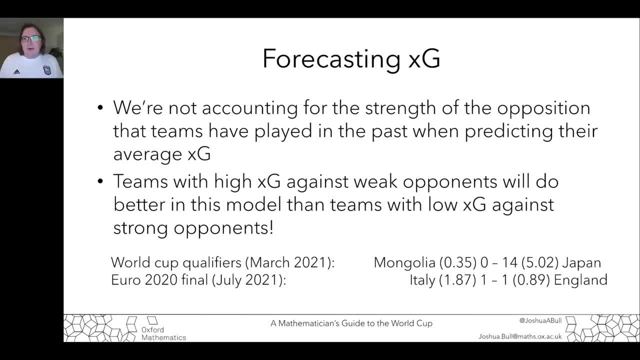 XG as England did. But on the whole we don't want to say these matches are comparable. You know, England scoring 0.9 XG against one of the strongest teams in the world is probably not the same as Japan scoring 5 XG against Mongolia. 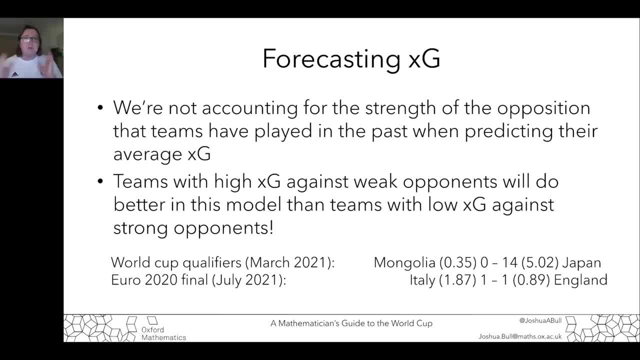 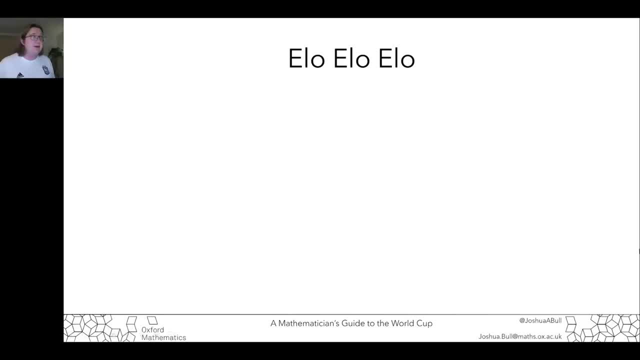 So maybe we don't want to just kind of crudely average these things and say, yes, Japan are a better team than England are. So I want to look at a way of measuring the relative strength of teams, and something which is very convenient is that this already exists out there. 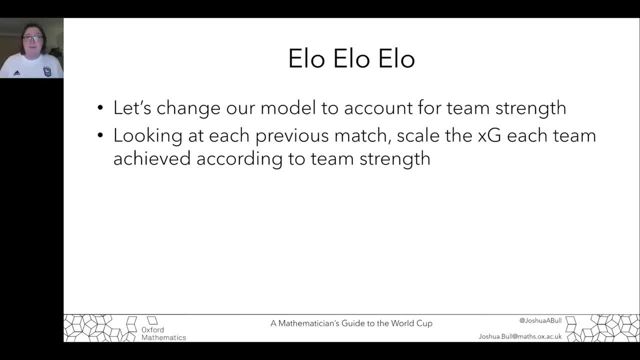 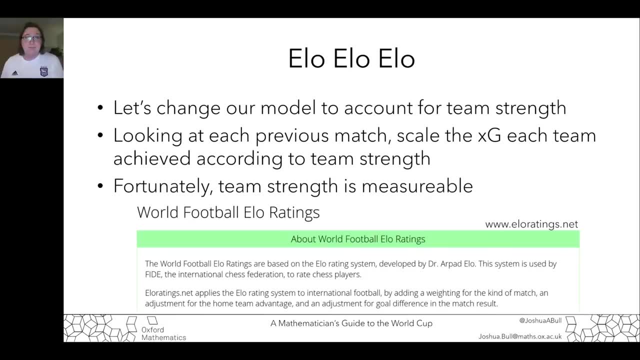 So what I want to do is scale the XG that each team is getting according to the strength of their opponents, And we can measure that, And I'm going to use this website, eloratingsnet, where basically they've been tracking football ratings for a very long time. 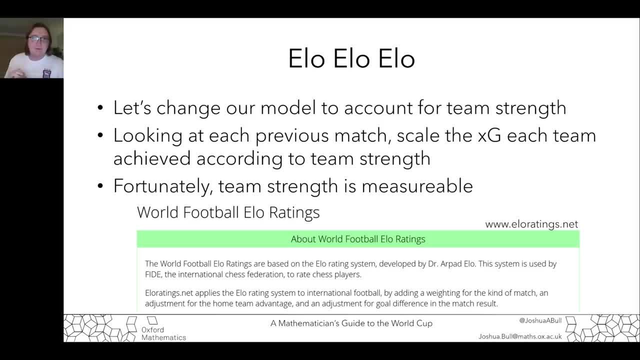 And you can go through and see exactly how they rank each football team on the international stage Against one another at any given time in history. And this is based on the way that chess players are rated: If a strong chess player loses to a weak chess player. 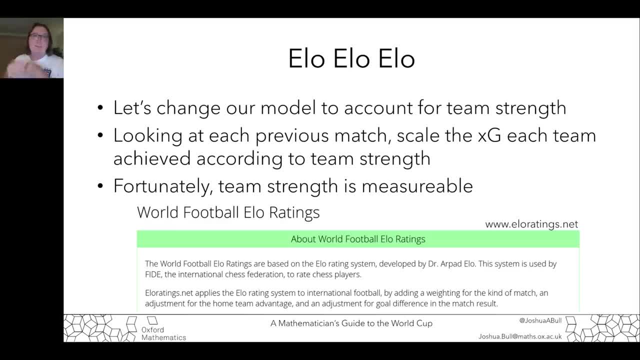 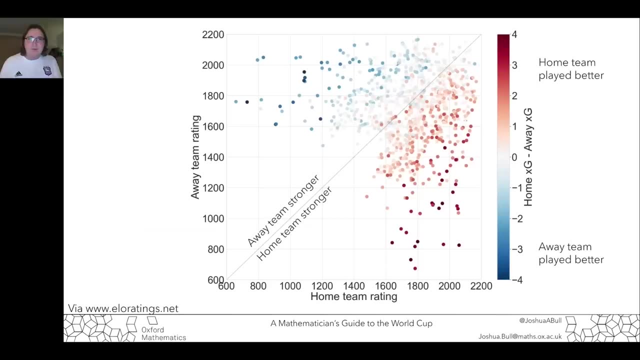 they drop down the rankings And it's exactly the same here. You get points for beating people that are stronger than you. lose them for losing to people that are weaker than you, or whatever way around that makes sense. So we can look at these ratings and assign a team strength to each team. 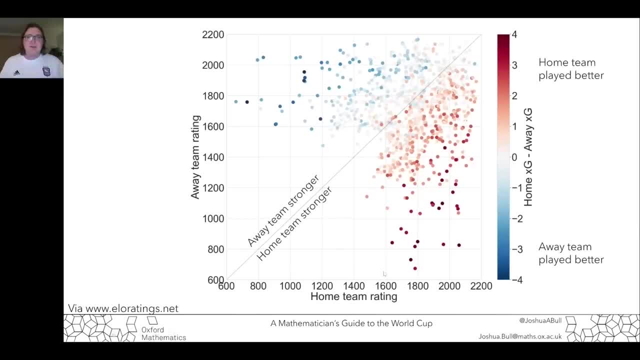 And it turns out when you do this you get some very pretty pictures. So what you're seeing on the bottom here is the home team rating. So the further towards the right we go, the stronger the home team is. Away team rating on the vertical axis. 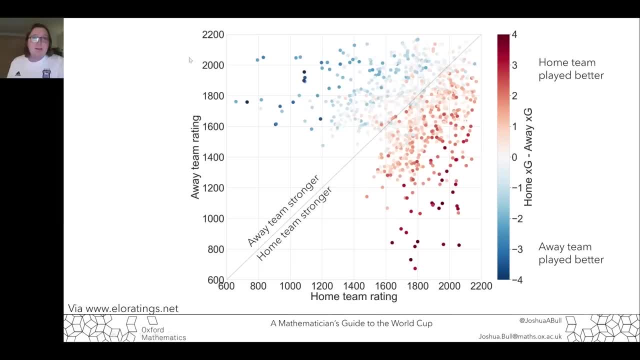 the further towards the top we are, the stronger that team is. So if we're in this kind of top left quadrant, Can you have a top left quadrant of half? I don't know, In this kind of top half the away team is stronger. 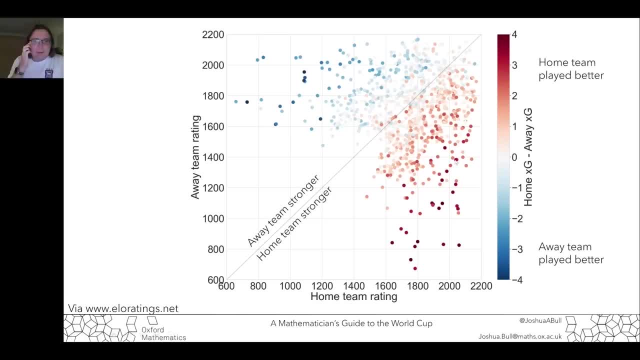 In the bottom half the home team is stronger and you can see that the way I've coloured these points is according to the difference in the xg between those teams. so if we see a red colour, that means the home team racks up more xg in that match than the away team. vice versa for a blue colour. so, conveniently, you. 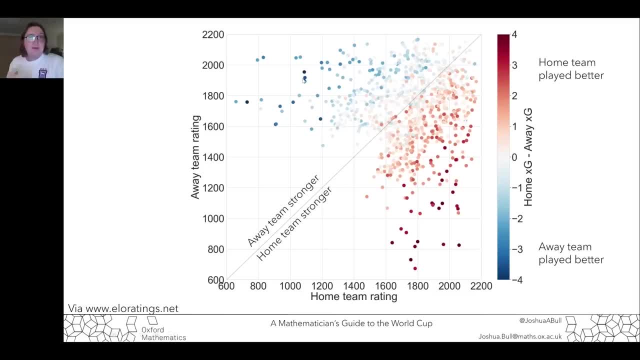 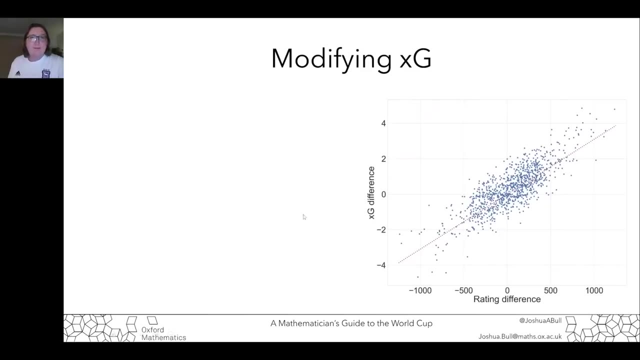 can see if the away team is very strong and the home team isn't, the away team scores more xg. that's kind of what we expect. this is a good sign. but you can also see it looks like it's making a very nice pattern indeed for us and in fact, if I plot the the difference there, the home xg minus. 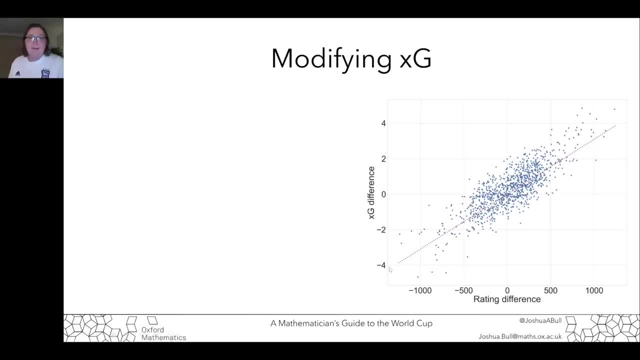 the away xg against their rating difference, we get a lovely straight line. so this basically gives us a way of saying: if team a is 500 elo points stronger than team b, we're expecting them on average to finish the game with 1.8 more xg or something along those lines. so this is a nice simple way of of converting. 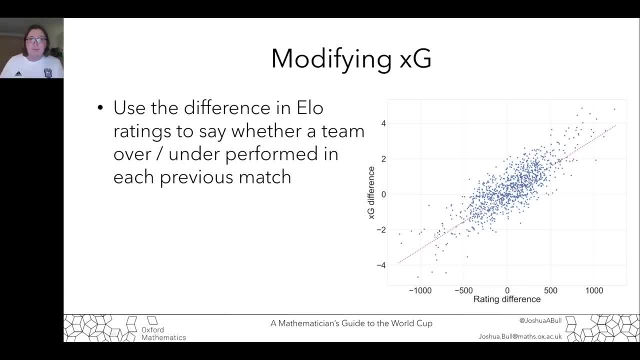 from the rating difference between two teams to the xg difference that we're expecting to see in there. so what I'm going to do now is adjust these previous xgs- the ones that I've put in my model since 2018- and I'm going to adjust them based on the rating difference between our teams. 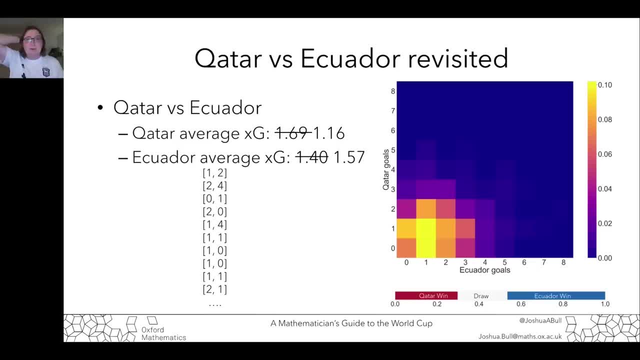 and you can see. coming back to Qatar versus Ecuador, this makes quite a big difference. so Qatar's expected xg has dropped down to 1.16, whereas Ecuador have gone up a bit to 1.57, and suddenly, when we simulate this game, many, many 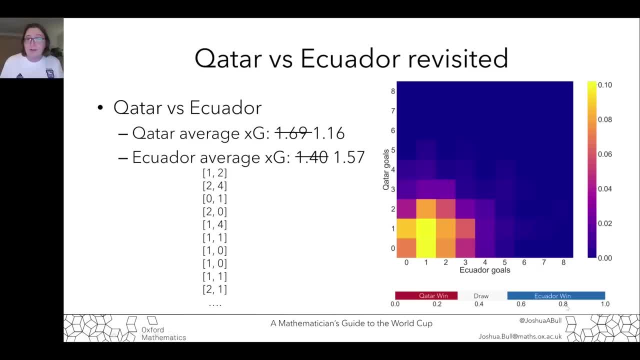 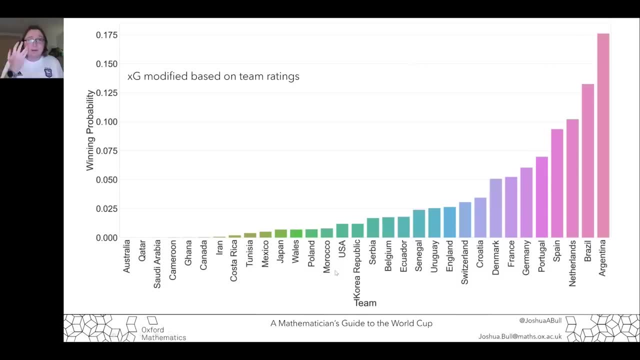 times. we see that actually Ecuador are more likely to win- up to 45 percent, Qatar down at 30 percent. so the tables have completely turned and we can return to our entire entire tournament and we see that we get something that's a little bit more believable than the xg that we've had in the 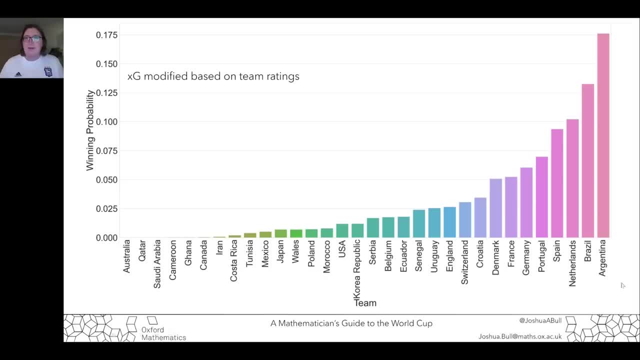 last couple of years and that's the reason why we're expecting to see a lot of xg drop down to the average football fan on the street. so at the top, teams like Brazil, Argentina, the Netherlands are expected to do very well and teams like Japan have dropped quite a long way down our 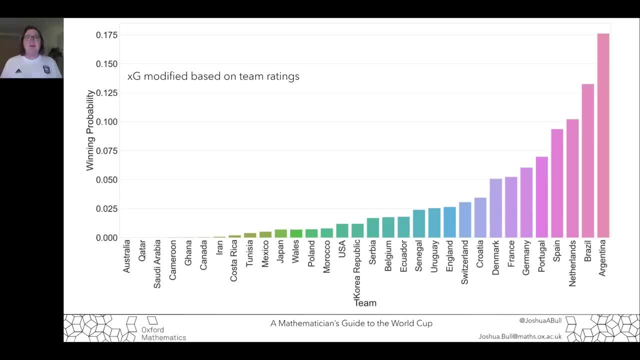 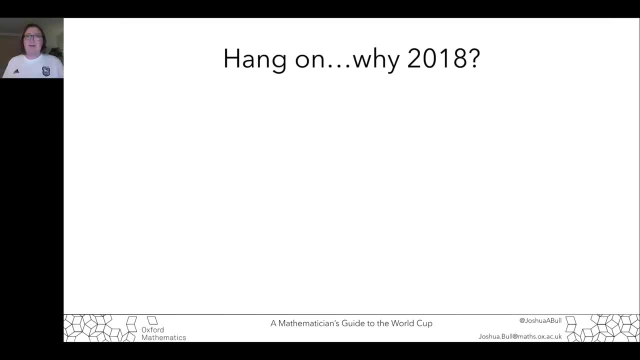 down our predictions, down our rankings, so much more believable. and we're done. right, hang on a minute, we're not done. why 2018? well, I chose 2018 for the very scientific reason that this is when England suddenly became good at football. um, and that's probably not a good. 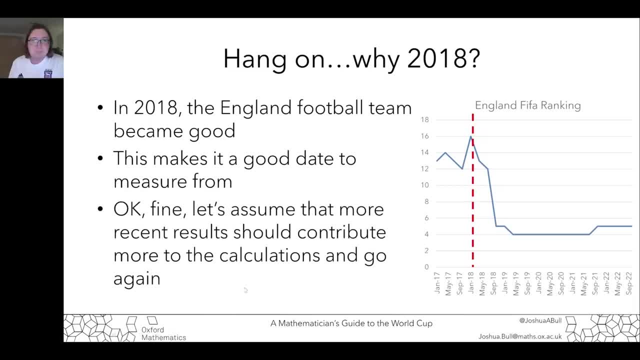 date to measure from you know that's very arbitrary and actually a lot of football fans will be keen to tell you that form is incredibly important and that the way a team has performed recently will be more predictive of what's about to happen. um, certainly when it comes to international 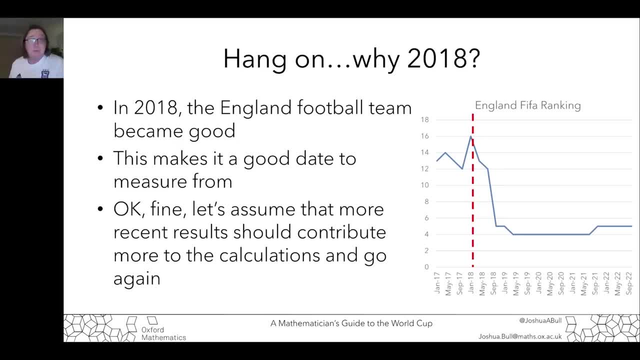 football. maybe the teams look very different now to how they looked four years ago, so it's probably a reasonable thing to say that more recent results um should be more important when we're making our predictions than results from two, three, four years ago. so I'm gonna, um, I'm gonna. 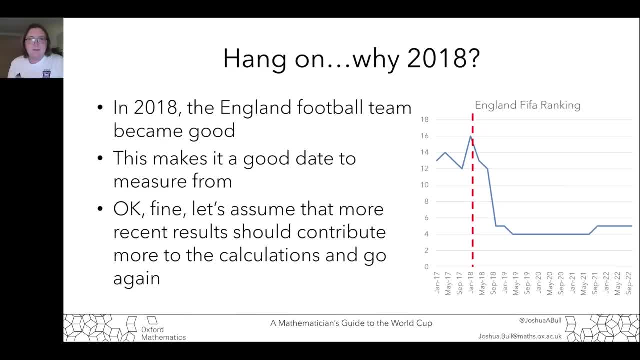 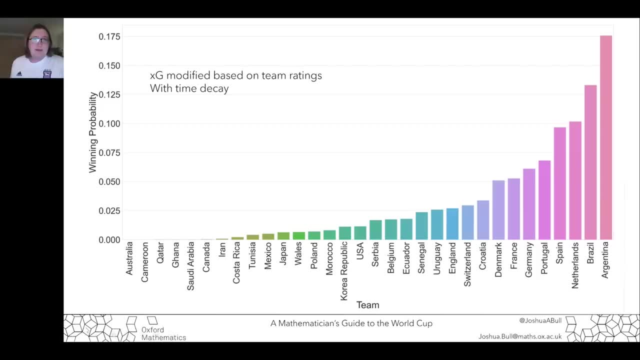 weight our results differently so that the more recent that result is, the um, the more credibility we're giving to it. when we calculate our averages, and when I include this kind of time decay, actually we end up with something quite similar again. um, you get a bit of shuffling England. 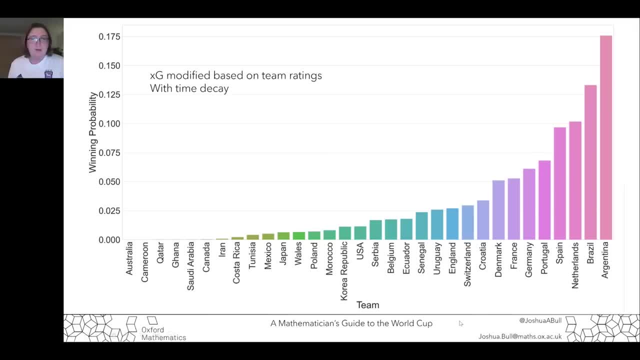 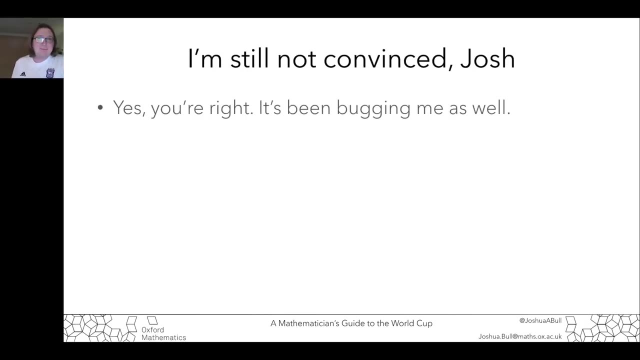 above Uruguay, which is, um, you know, probably good. let's hope that that happens, um, but we're still not far enough up this table for my liking, and you know really, um that, whether that means we should challenge some assumptions. I'm going to, and, in fact, what assumptions could we change? well, 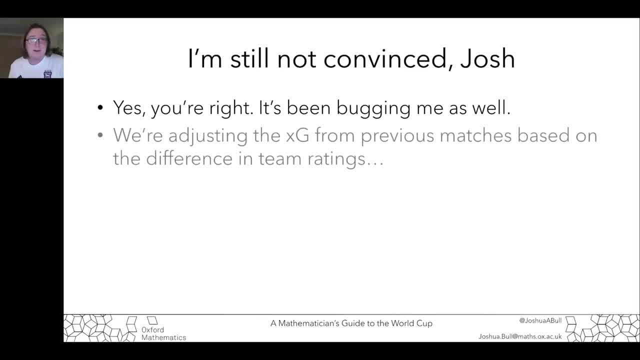 there is something that we've been glossing over quite a lot. we're changing the xg from previous matches based on how different the team matings are, but I'm not actually using that, so I'm calculating what I think the xg is going to be. 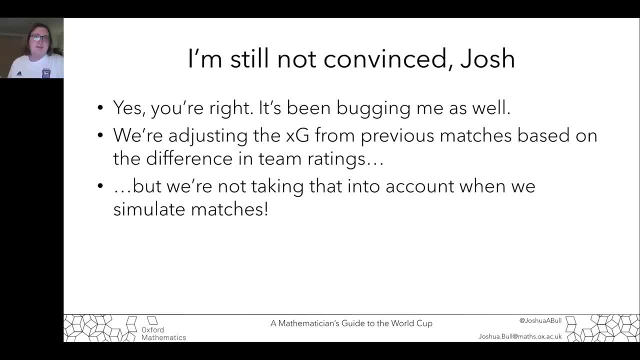 for a given team, and I say Qatar's xg on average is 1.4, and so I say they're likely to score 1.4 goals per game, whether they're playing Brazil or whether they're playing Ghana. so that's probably not good. we probably want to be adjusting our matches based on who they're playing rather than 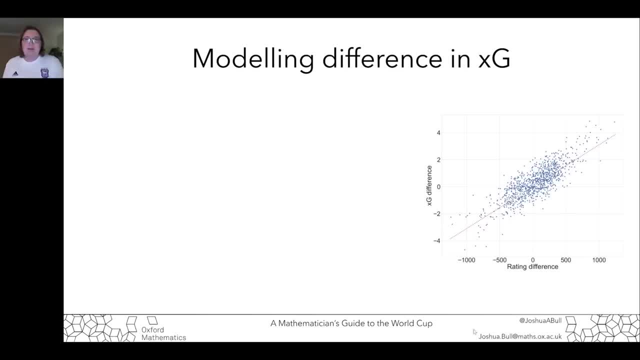 just based on who they've played in the past. and in fact, if we come back to this um nice straight line that we saw earlier, well, we can just sample directly from this. you know, if we have a 500 point rating difference between the teams, why don't we just sample that they should have an xg difference? 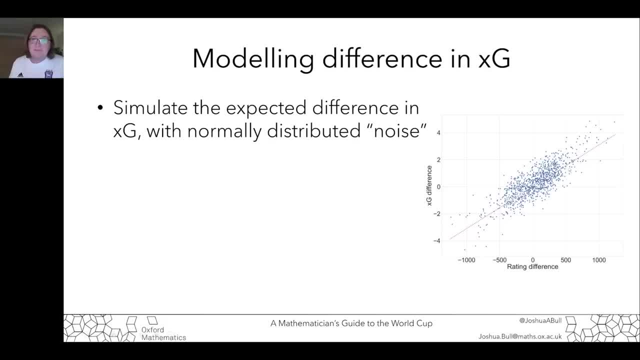 of 1.8 or whatever this red line is, and in fact this is um a lovely, a lovely normal distribution around this line, um, and so in fact we can not only take the mean value, but we can also add that noise in and get a sense for. 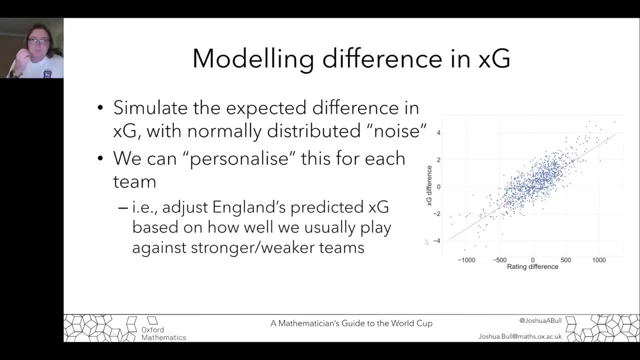 the kind of width of this distribution here, and in fact we can personalize this for each team so we can look at each team and see um on average when they play an opponent who is stronger or weaker than them. what do we expect this xg difference to be? and this um seems to. 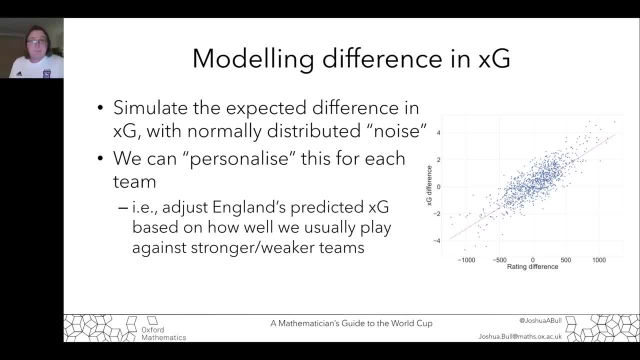 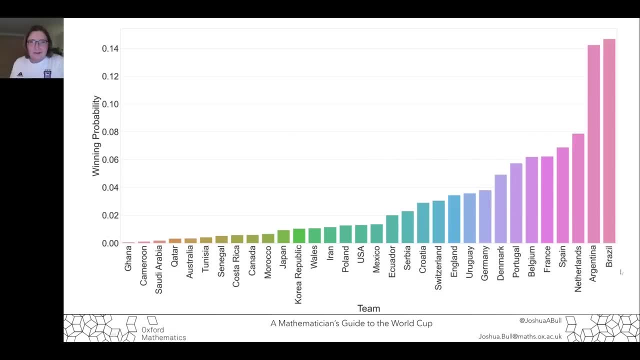 be quite a nice simple model that is, uh, quite good at predicting the data that we can see, in the past at least, and you can see here. this gives us a very similar ordering in terms of Brazil, Argentina, Netherlands, Spain. the teams that that we think are likely to be good are up at the top. um, England's. 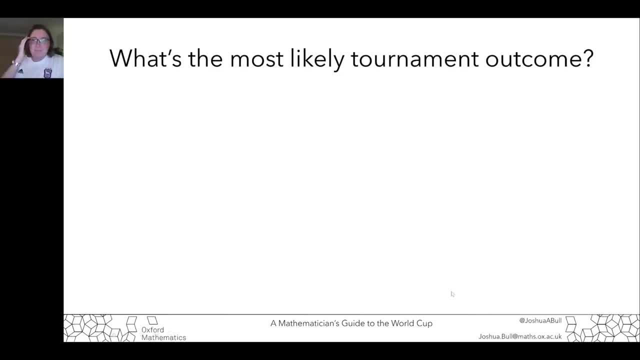 still depressingly low in this model, um, but we can use this then to actually look at what we think the most likely outcome of the tournament is. so the way we're doing this is for each match, just to estimate the difference according to elo ratingsnet. I'm going to use that to predict the difference. 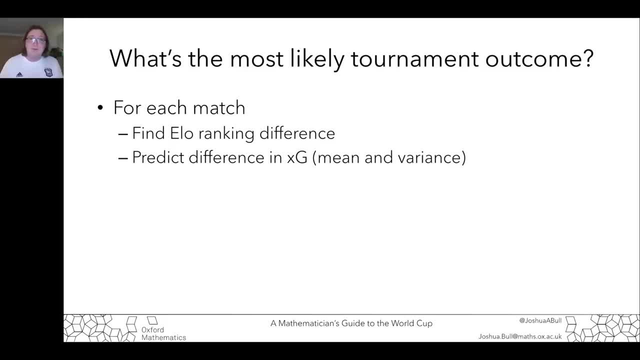 in xg between those teams and I'm going to sample from some distribution with that mean and variance. and when I do that, that will say, for this version of Qatar versus Ecuador, we're expecting Ecuador to be 0.3 xg ahead. and then I'm kind of doing some fudging based on their- uh, their previous xg values. 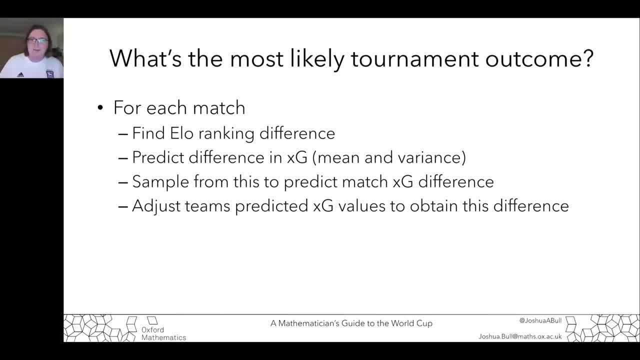 to kind of scale them so that I get the difference that I'm expecting to see. so there's a bit of fudging going on in there and I then sample from those two Poisson distributions for those given xg's to get the right score, um, or the predicted score. and again, we repeat this a lot of times. 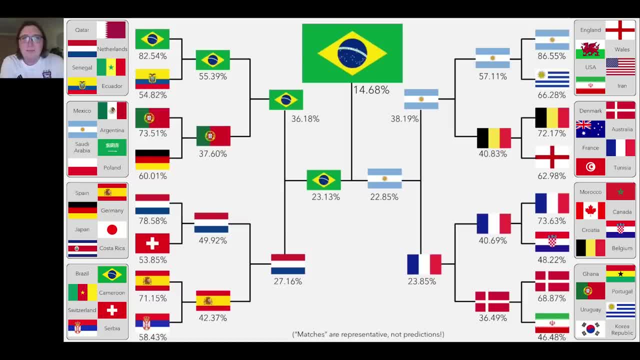 and this is what comes out. so this is, um you know, my uh, my prediction, my uh- future in sports modeling on the line. um, my model is basically saying that, um, Brazil are definitely looking most likely to win, but by no means guaranteed, so it's putting them at around 15. 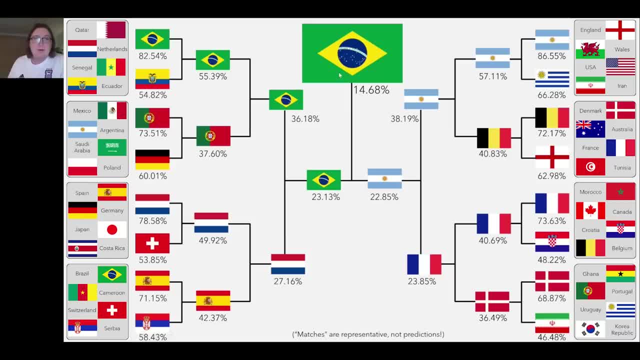 percent of my simulations they've come out on top and what you're seeing here, um, really is just showing who I think the the two teams who appear in the final most often are the four teams in the quarterfinals and so on. so I'm not saying that I think this set of matches is the most likely lineup. 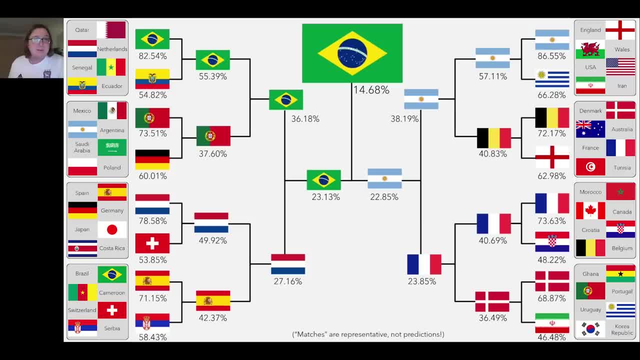 and I don't actually know if it's possible to get these matches, given the the group stages, um, but we'll see how that goes. We will, uh, we will see. so you can see that England, at least, are favored to make it out of the groups in 60 of the simulations and actually in this model they are, they are. 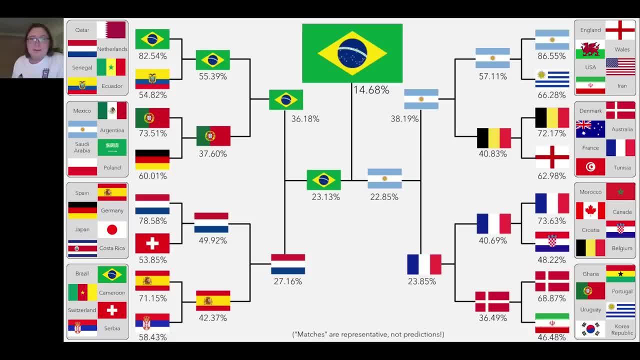 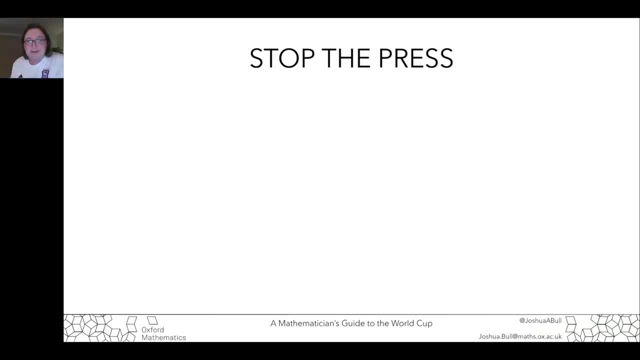 quite close as we go further and further through. so you know we're maybe not completely out of the running yet. um, hang on, stop the press. there's one more change, one last minute change to our model that we can make. so we've not included the FCH factor at all. 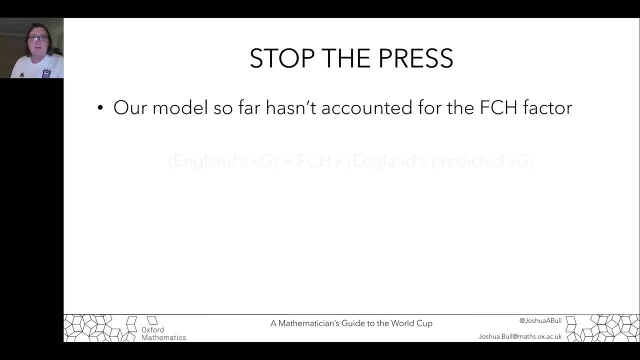 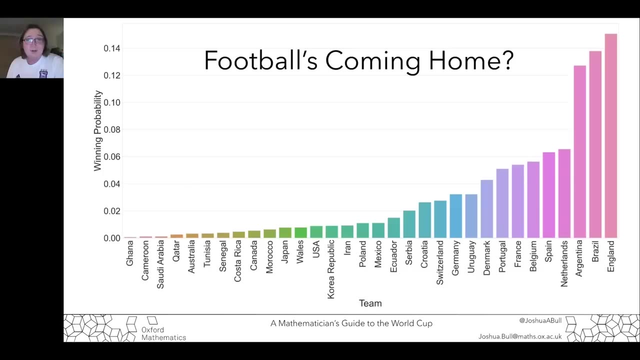 um. so the FCH factor is a technical mathematical term for those who aren't familiar with it- um, and this is a value which scales the England team's xg based on whether or not football's coming home, and you can see that the FCH factor only needs to be about 1.7 in order for England. 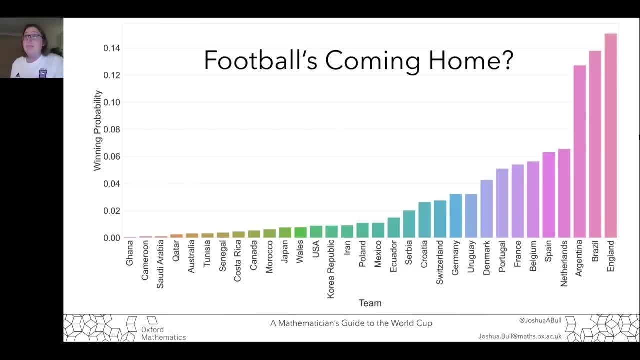 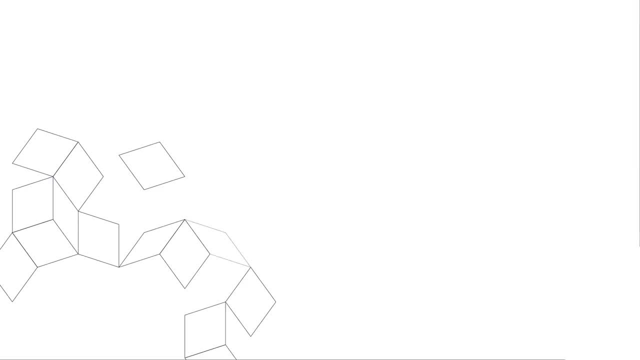 to uh, to top the table. so you know, it's not unlikely, it's not unlikely, it's quite unlikely. that that's the FCH factor and that one would be a good thing to know. So it's really just a long way off. so there's a lot of uncertainty in terms of what's going to happen. and that's why we've been here and what we're doing, and we'll speak about that. but the big issue is it's not out of the group and it's not out of fans and and the game is out there. so I was thinking that, like maybe we should, we should add in some of the things that we've talked about. today. so maybe the only thing that needs to be done is to get the teams to come out and say: hey, what do you think this is? you've got a good idea of what's going on with this. you know we're not doing it right now, we're not going to go into it, but the problem is if it's a good idea or not. we're going to. go ahead and get it done.